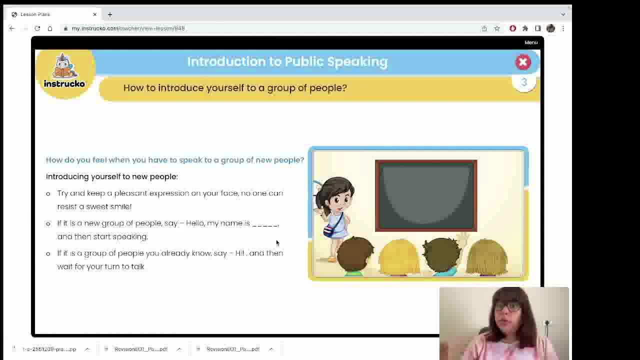 to a group of people. You tell people what your name is. Maybe you know the people who you are speaking to. They might want to know where do you come from, which school do you study in, So you can tell them that kind of information. okay, Now, if it is a group of people who you already 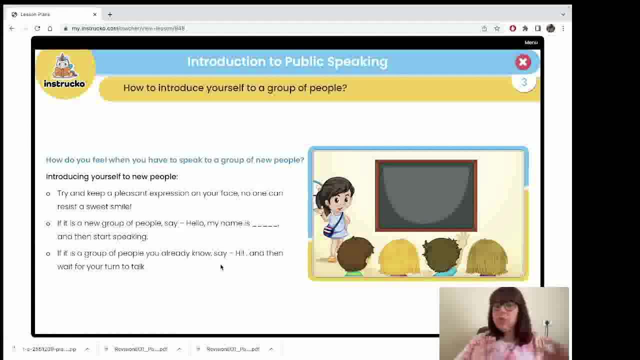 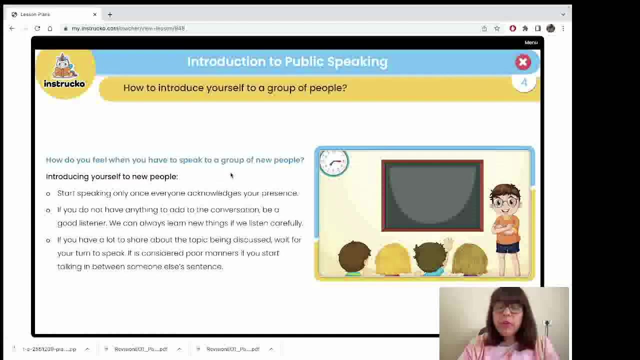 know and you want to join into the conversation. should we just go and start talking in between the conversation? No, we mustn't. okay, We must wait for our turn to speak. okay, We will say hi, And then we will wait for our turn to speak. okay, That works Amazing. Now how do you? 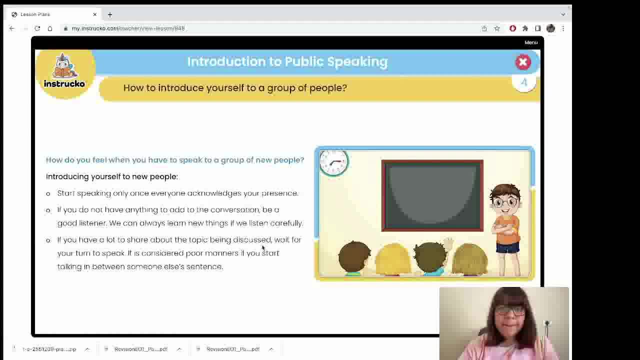 feel when you have to speak to a group of new people? Do you feel nervous Sometimes, do you feel a little bit underconfident? Okay, So we are going to work around all of those issues, okay Now. firstly, you start speaking only once every two or three months. okay, So you start. 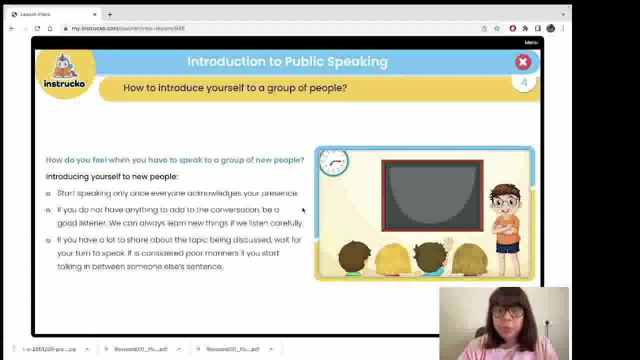 speaking only once every two or three months. okay, So you start speaking only once every two or three months. okay, So you start speaking only once every two or three months. okay. Also, you start speaking only once. every one acknowledges your presence Once everyone. 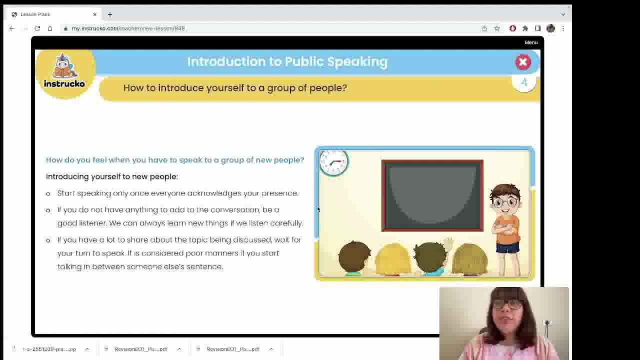 says hi to you, then start speaking. Or if you see that you know someone hasn't noticed your presence, someone hadn't noticed that you've joined in the group, say hello to them. okay, Say hi to everyone and then start speaking. That shows the people in the group. 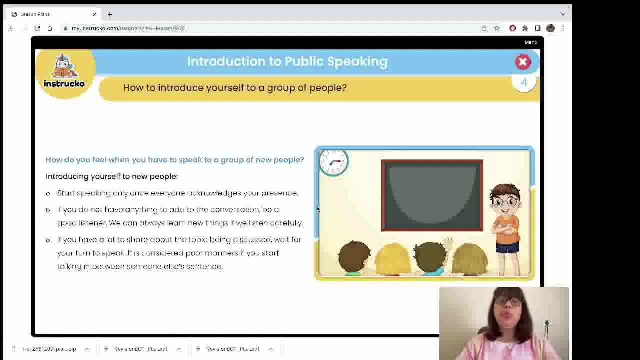 that you really care about all of them and you really care that they listen to what you are saying. okay, So, when you say hi to everyone, when you establish your presence in the group, people will listen to you carefully. okay, So, if you chat up to one Another, people actually do so and it works. okay, Now this works. 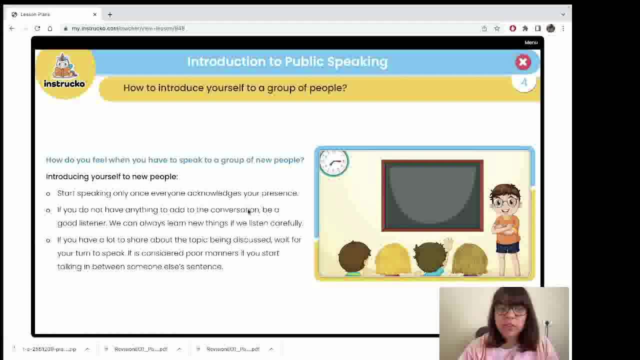 if you do not have anything to add to the conversation, be a good listener. we can always learn new things if we listen very carefully. yes, listening carefully is a beautiful thing to do. you learn so many things, you know, if you just listen to people talking around you. 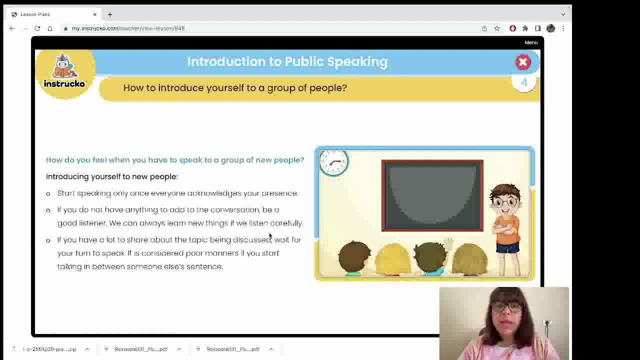 yes, maybe you know someone can be having a chat. two of your friends might be having a chat about a new say science project. they tried together. yes, and then what do you do? do you listen to them or do you try telling them about your thing that you have come to say? of course you listen to. 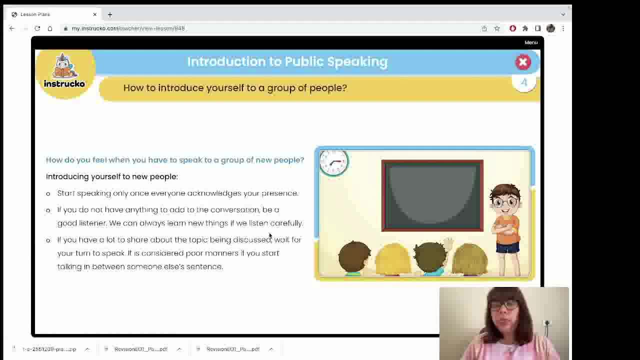 them, then you never know, tomorrow even you know how to you know, do whatever they were doing. maybe they built a beautiful volcano together so you can listen and pick up all the ingredients of the volcano. you can learn how to build the structure of the volcano. yes, so listening, again like speaking in, is an art. you have to listen very carefully and only then can. 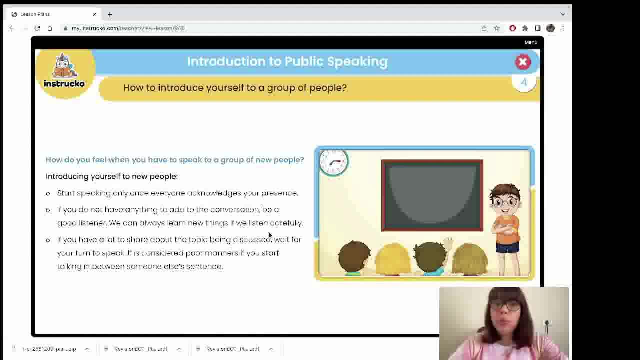 you pick up new information around you. so if you go into a group of people and you have nothing new to add to the conversation and if you think they are having a beautiful conversation, listen to them. yes, okay, now, if you have a lot to share about a topic being discussed, now we are going. 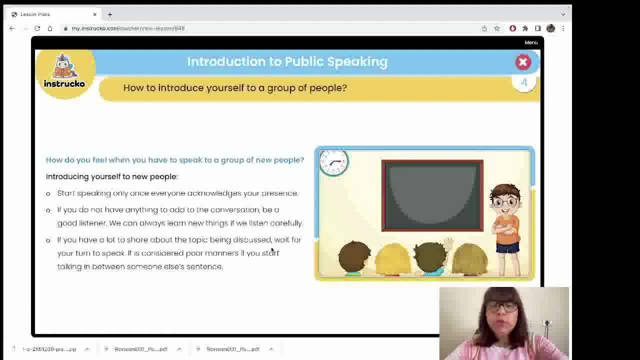 to the other end of the spectrum. so in the first scenario you didn't have anything to add on, so you stay in and you listen. now, in the second scenario, you have lots and lots of information to add on to what is being said already. maybe it's about your favorite. you know superhero and you know. 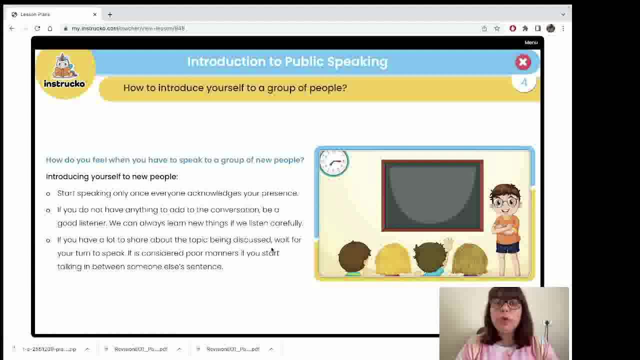 all about them and you want to talk a lot, a lot, a lot. so what do you do? do you hold on, do you hold your horses, or do you just jump in and you override everyone and start speaking? very good, you just wait for your turn and then speak. 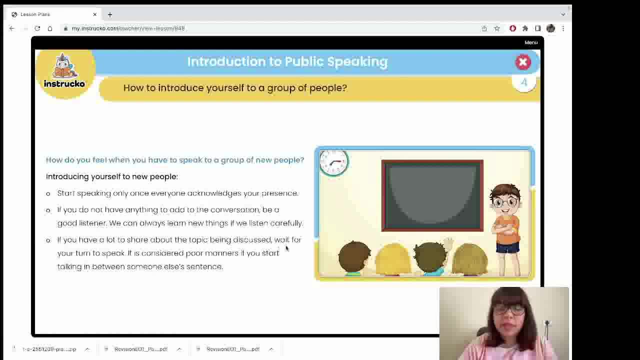 okay if you have a lot to share about the topic being discussed. wait for your turn to speak. it is considered poor manners if you start talking in between someone else's sentence. okay, so we must wait for the other people to finish saying whatever they are saying and then we come into the 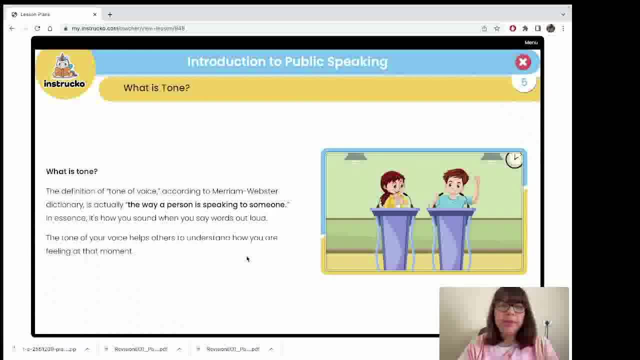 conversation, okay, wonderful now. so today we are going to talk about something very, very important. have you ever heard of this word called tone? tone, can you say it with me? tone, very good. so what is tone? do you know already? okay, if you don't know what tone is, I'll tell you today. okay, the definition of tone of voice according to the. 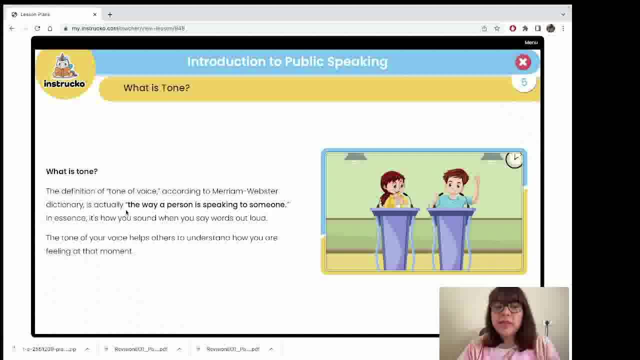 dictionary is actually the way a person is speaking to someone. the way you sound when you speak to someone is your tone of voice. so the way a person is speaking to someone is your tone of voice. method of speaking in a geral tone more Или diksa voor die Trinit- tone or voice. okay, in essence it is. 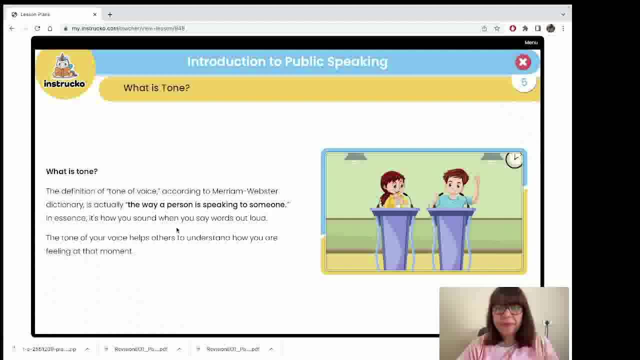 how you sound when you say words out aloud. so when I say, hmm, who speaks in a a very sweet tone, then you think of someone, maybe your mother, maybe your aunt, maybe your dad. yes, there is always. you associate different tones of voices with different people. if I say who speaks in a very grumpy tone, 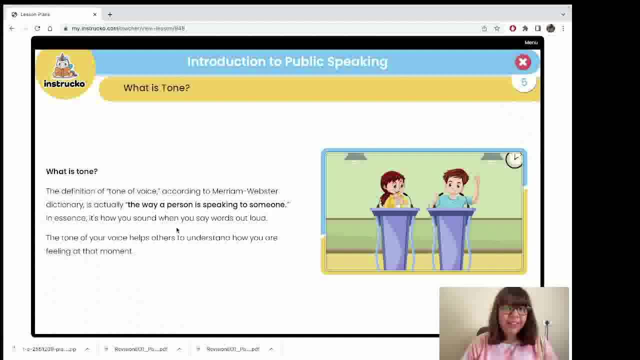 maybe your dad? yes, so there is always. you know, you associate different tones of voices with different people. if I say, who speaks in a very grumpy tone, maybe associate it with someone around you. yes, okay, who's always sad? who always speaks in a sad tone? yes, you have someone in mind, right? so the same way, everyone else hears the way you speak and 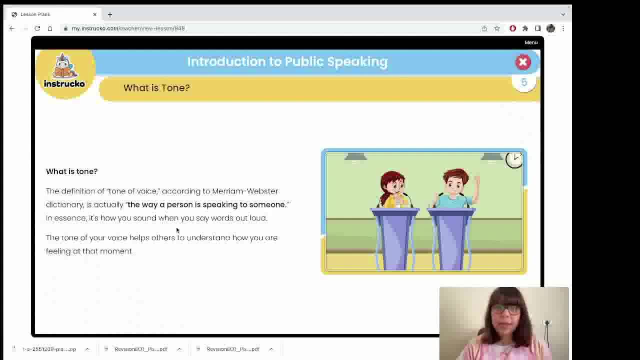 they associate you with a certain tone of voice. okay, so how would you like your tone of voice to be? would you like it to be beautiful and sweet and happy, or would you like it to be sad and sullen, or maybe a little grumpy? of course we should try and sound happy in general, if not. 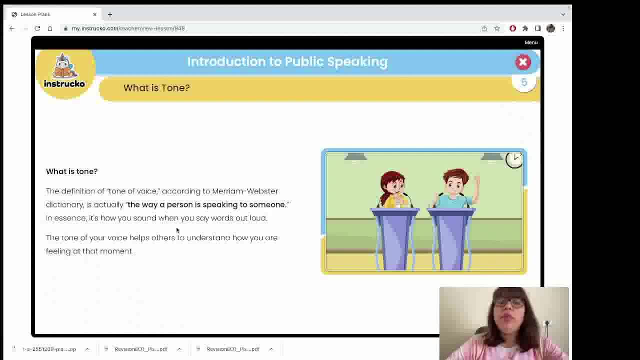 happy. we should try and sound pleasant. okay, our tone of voice should be pleasant. it should be confident. yes, okay. now the tone of voice. it serves another purpose. okay, apart from adding on to your personality, your tone of voice serves a second purpose which is very, very important in public. 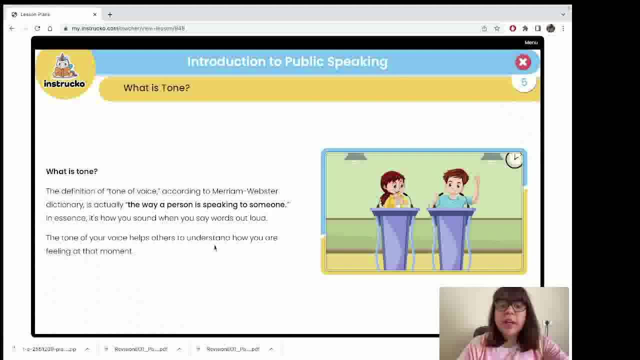 speaking the tone of your voice, helps you to be happy, Helps others to understand how you are feeling at that moment. Okay, so imagine you walk into a room and your mom says: Hi, Aditi, how was your day Then? what do you think? 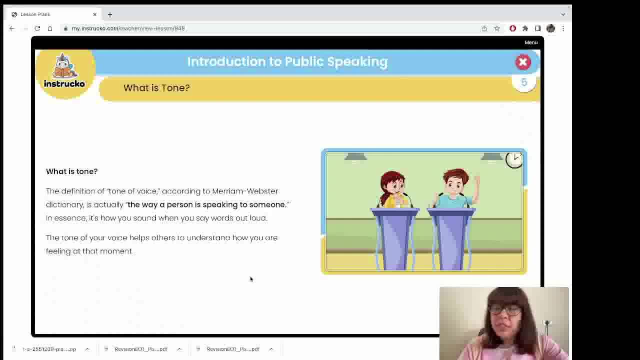 How's your mom feeling at that point? Yes, she's feeling a little sad, maybe. And then now cut to the second scenario. You walk into the room and your mom says: Hi, Aditi, how was your day? Then you know, mom's been having a great day, right. 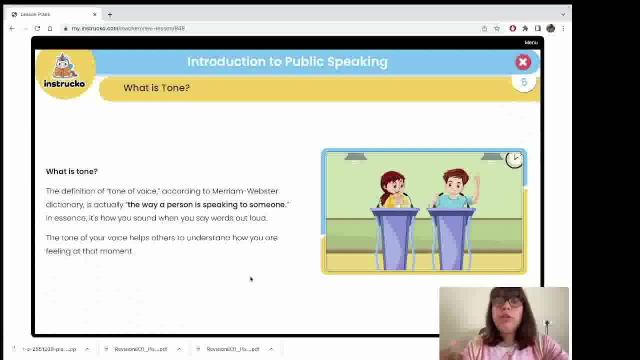 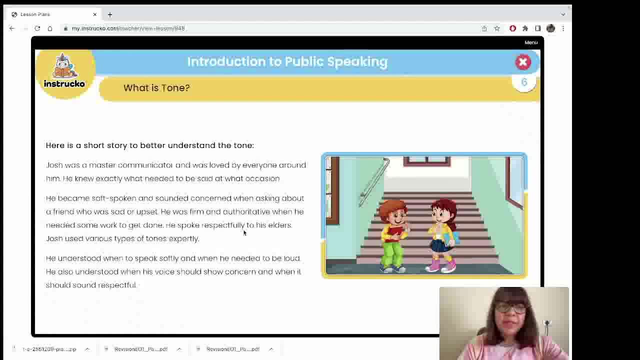 So your tone of voice serves another purpose when you speak to other people, It lets them know how you're feeling at that moment. Okay, Now, here is a short story to better understand tone. Okay, so we're going to talk about a little boy, Josh. 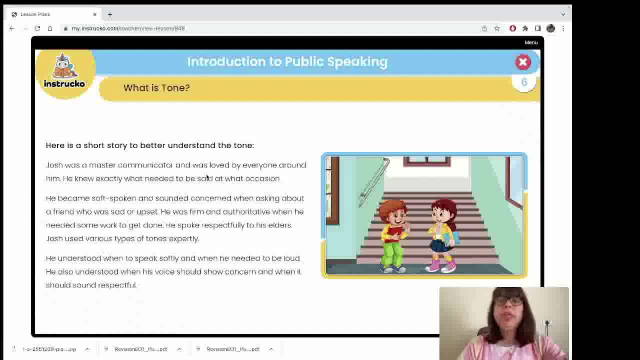 who knows to use his tone of voice very beautifully in different situations. So now we will try and listen to Josh's story And we will try and remember how Josh uses different tones of voices in different situations. Okay, Now Josh is a master communicator and was loved by everyone around him. 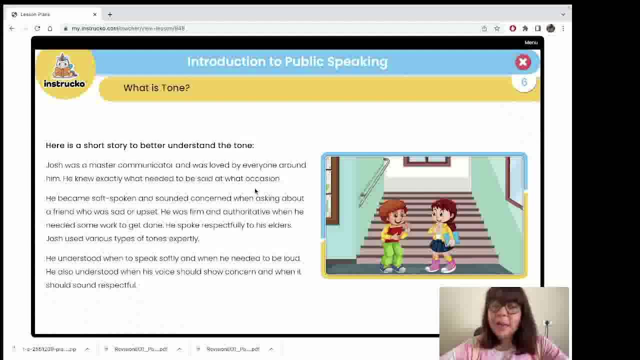 He knew exactly what needed to be said at what occasion. He became soft spoken and sounded concerned. when someone asked about a friend who was sad or upset, He was firm and authoritative. When he needed to get some work done, he spoke respectfully to his elders. 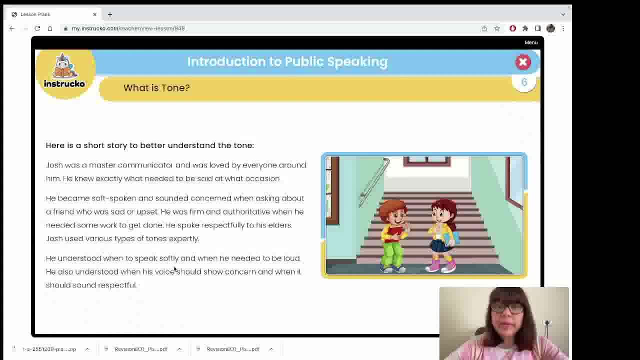 Josh used various types of tones expertly. He knew exactly what kind of tone had to be used in what kind of situation. He understood when to speak softly and when he needed to be loud. He also understood when his voice should show concern and when it should sound respectful. 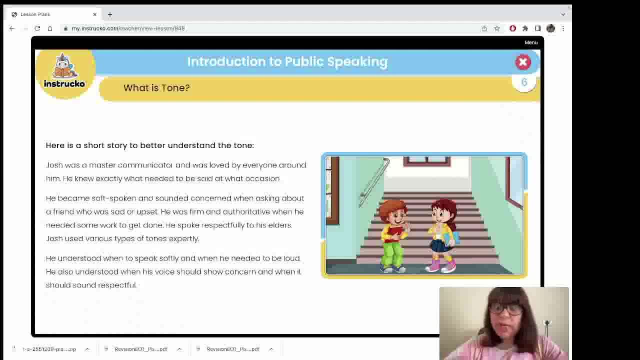 Okay. so let's try and be like Josh. Okay, let's try and use our tone of voice differently in different situations. Maybe you can try and practice this at home. Okay, maybe you know you go and tell your mama something in a sad tone of voice. 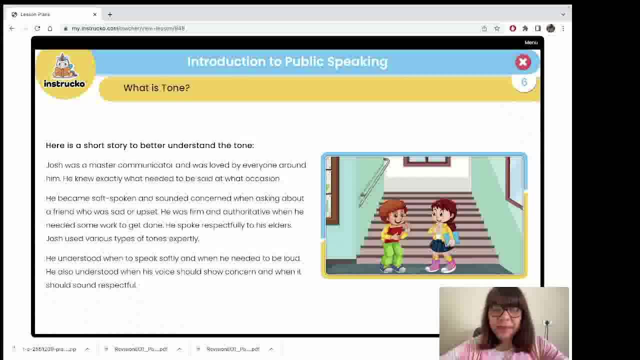 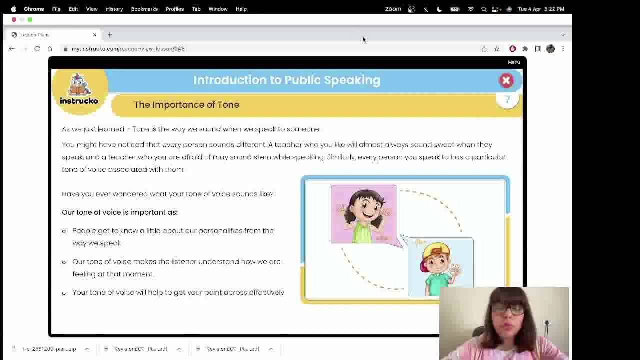 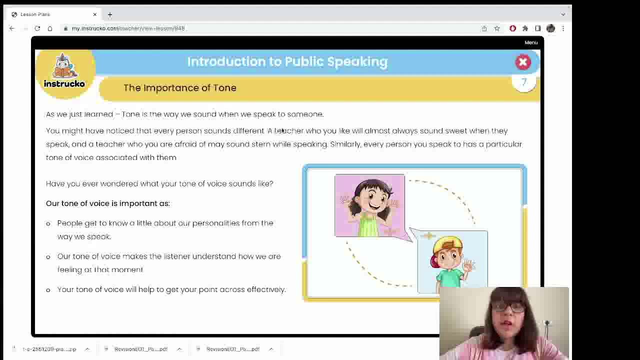 See if she understands in that moment if you're sad. Okay, so now we're going to talk a little bit about the importance of tone. Why is tone so important? Why is tone important? now, as We just learned, tone is the way we sound when we speak to someone. 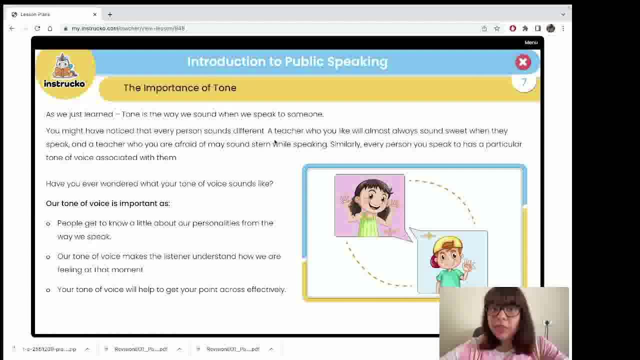 you might have noticed that every person sounds different. a Teacher who you like will almost always sound sweet when they speak. a Teacher who you are afraid of might sound stern. Stern means very strict while speaking. similarly, every person you speak to has a particular tone of voice associated with them. you relate to a 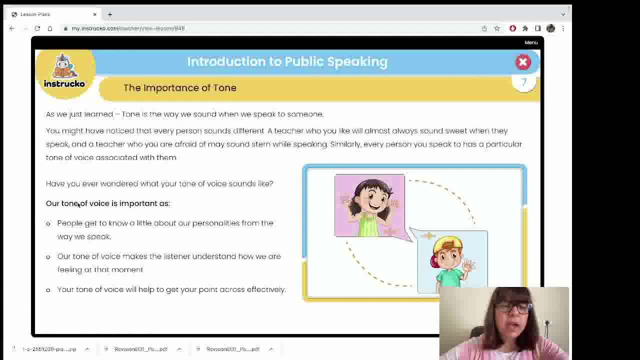 tone of voice with different people right now. have you ever wondered what your tone of voice sounds like to other people? okay, maybe you can find out. maybe you can go and ask around a little bit. your tone of voice is important, as people get to know a little bit about our personalities from the way we speak. 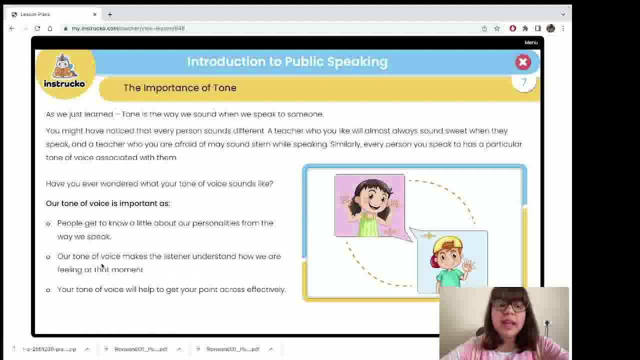 our tone of voice makes the listener understand how we are feeling at that moment. your tone of voice will help people to get your point. it'll help you to get your point across to people very, very effectively. yes, sometimes you just want to say very little, but you want to get your message across. suppose you know? 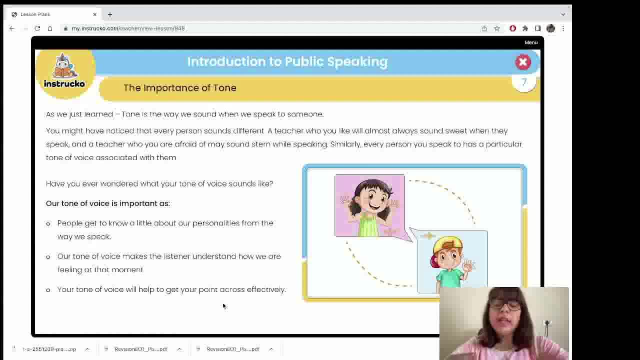 there is a child who's been bullying you in school and they've been pushing you around and one day you decide that you know, enough is enough. today I am going to end this. so when that child comes up to you, you just say stop, stop. today I am not going to take this anymore. there will be consequences if 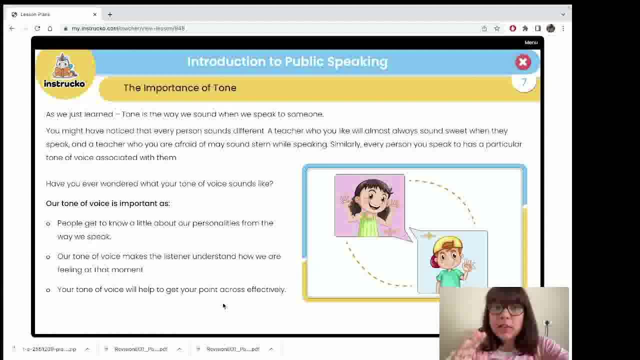 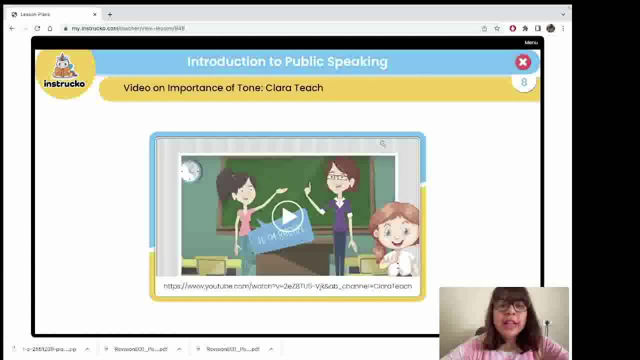 you continue like this, and if you say it in a stern, in a very firm tone of voice, that child will stop doing it again. you should try it, you know? okay, wonderful, thank you for listening so carefully so far. now we are going to end today's session with a very, very short video on why is tone important? 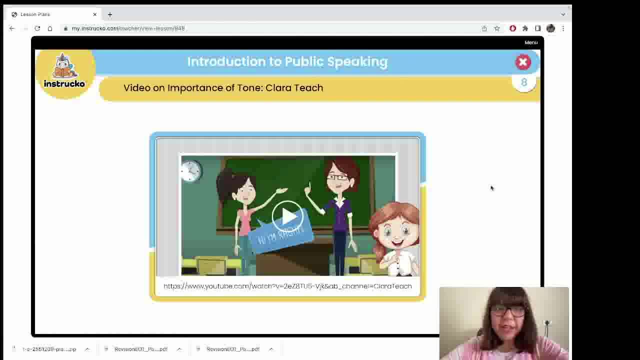 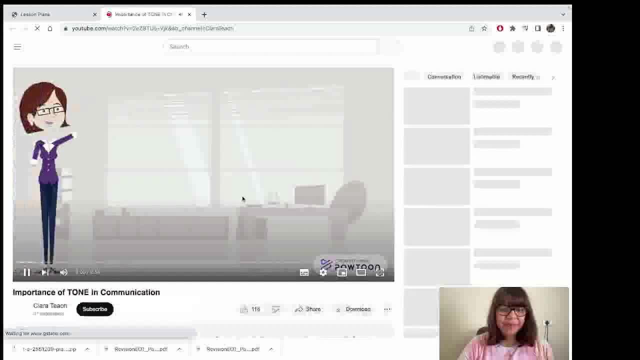 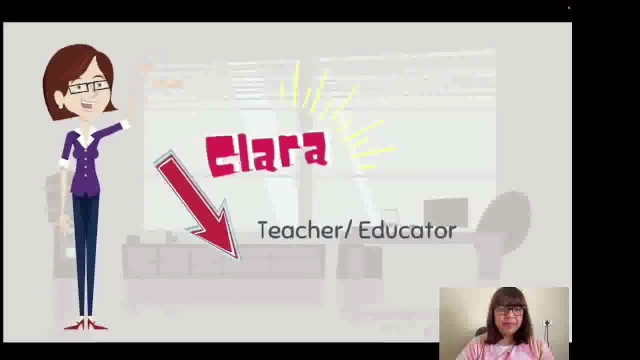 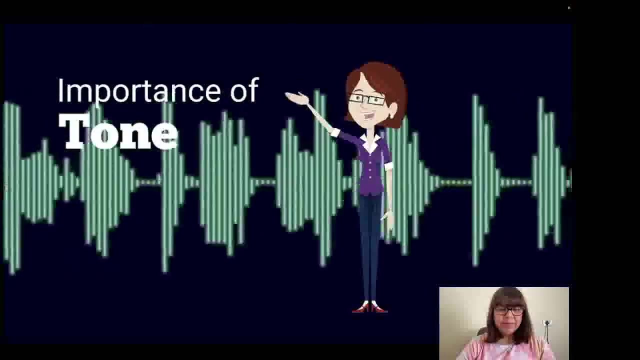 okay, so listen in carefully. are you ready for the video? let's start. hello everyone. my name is Clara and today we'll have a quick discussion on why is tone important? let's learn why our tone of voice is important to think about when talking to another person. imagine: 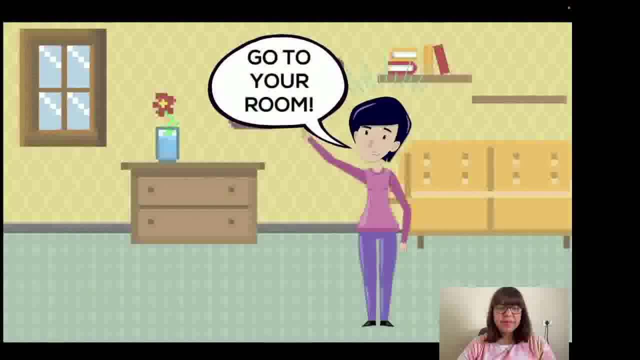 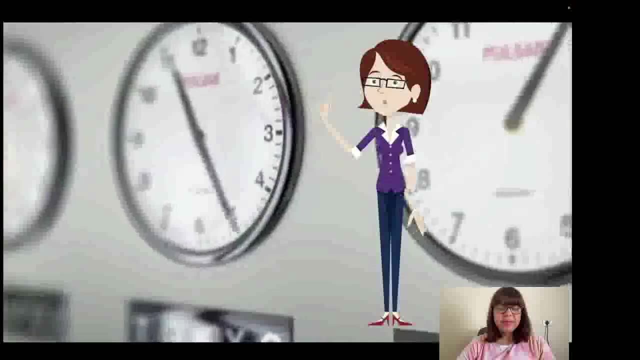 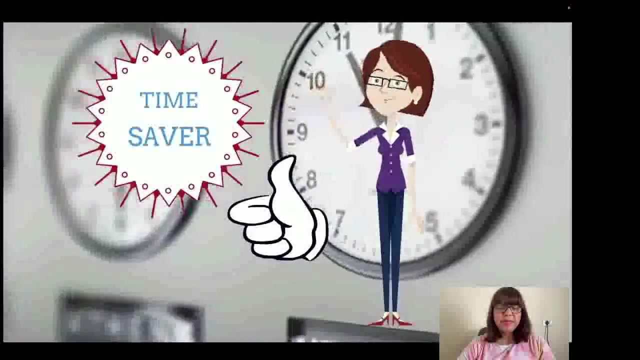 your mother telling you go to your room. hearing her say this with that strict tone means she is serious upset and that she doesn't want to hear any explanations from you. understanding someone's tone is a time saver. imagine if she needed to explain what she was feeling at that moment without using tone. it'll. 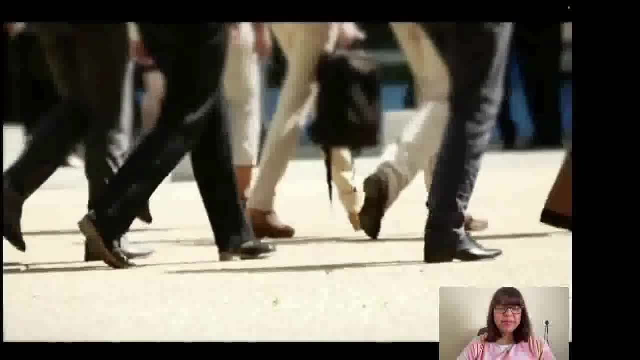 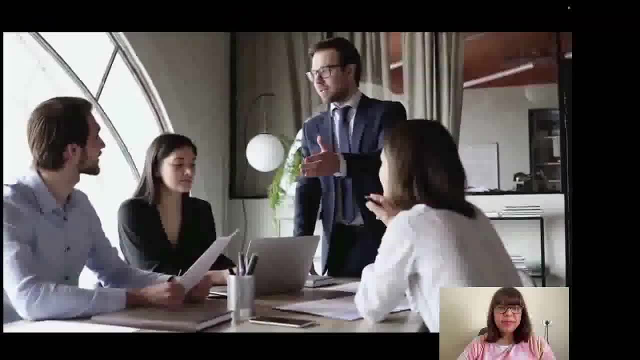 take her extra minutes to figure out who she was talking about, and they can use some hard work to get their thing done. if you can plan ahead, okay, thank you all. have a great day and have a great day. bye, bye. do so. Visualize a world full of people explaining everything without using tone. It will take. 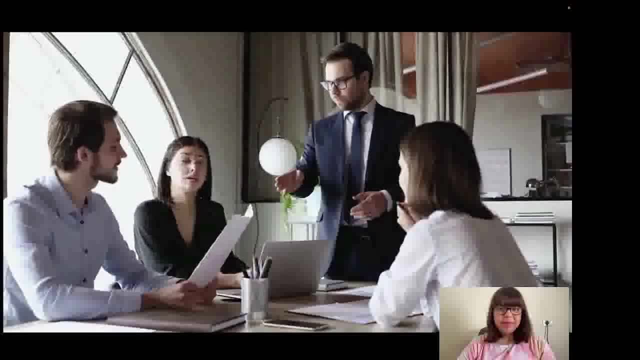 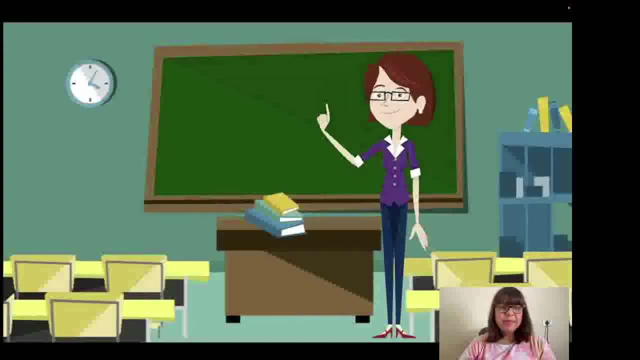 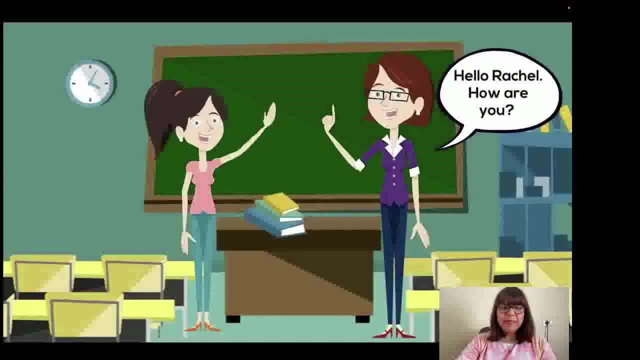 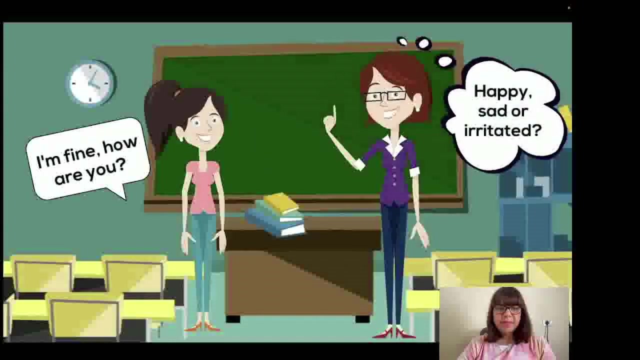 a lot of time and it will get very tiring. Allow me to show you another example. Let's have one person named Rachel say the same thing, but with different tones. I'm fine. How are you? Did she sound happy, sad or irritated? The answer is: happy. Take two. 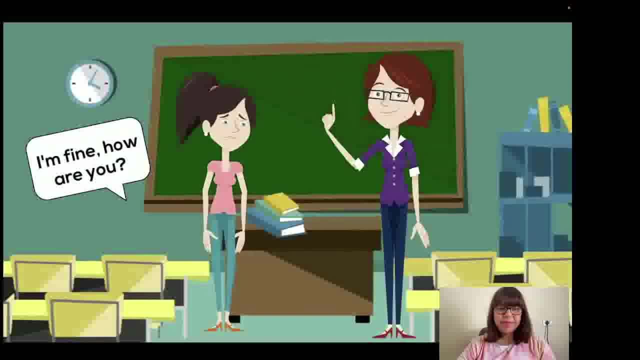 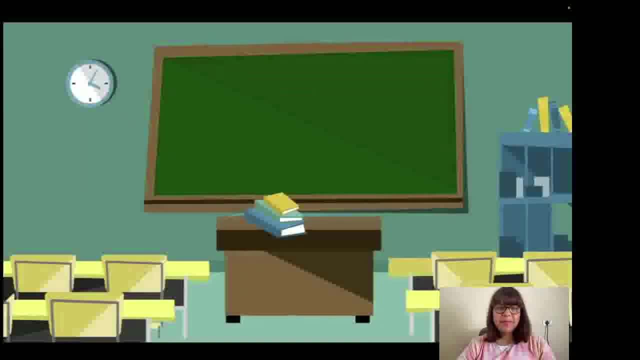 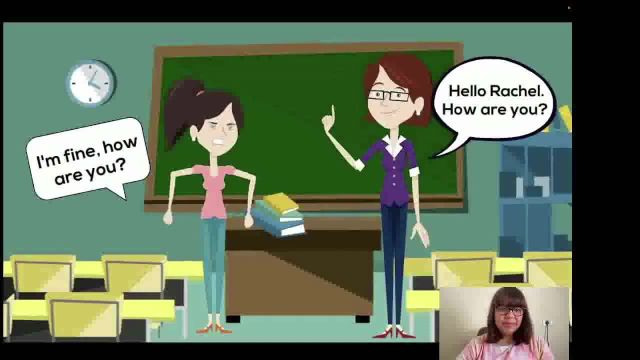 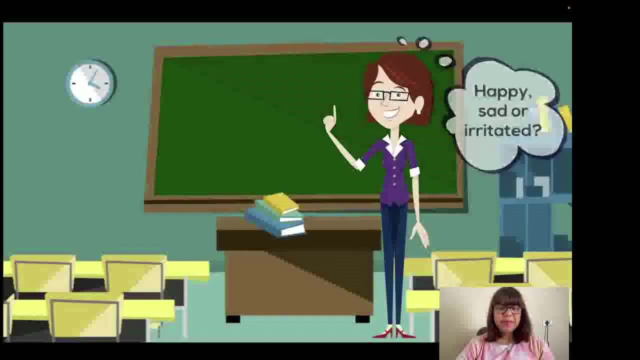 Rachel, I'm fine. How are you? Did she sound happy, sad or irritated? The answer is sad. Take three, Rachel, I'm fine. How are you? Did she sound happy, sad or irritated? The answer is: irritated. Picture. 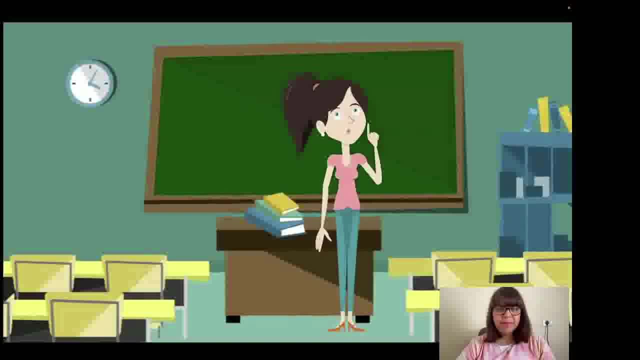 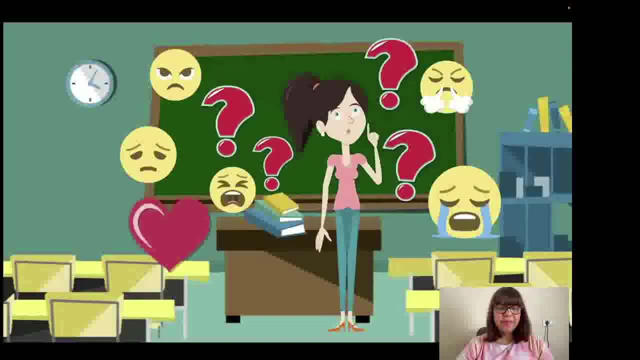 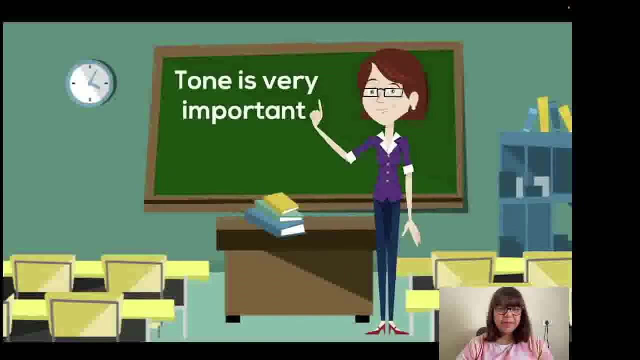 Rachel saying the same thing, but without the proper tone matching her emotion, We wouldn't be able to understand what is she really feeling. As you can hear, tone is very important. It helps us understand the emotion and intention of the people that we talk to. It's essential. 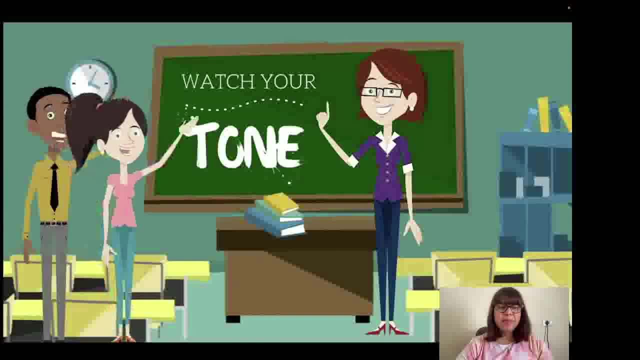 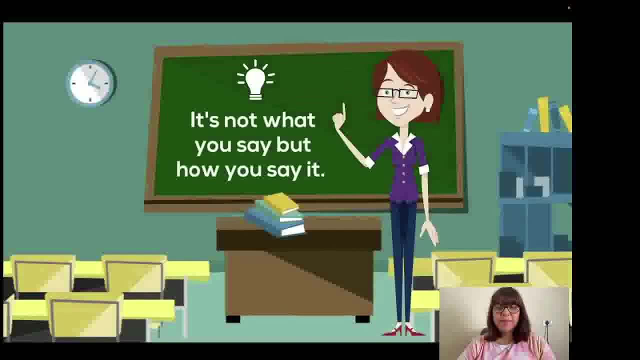 that we watch our tone because it affects the people around us. Remember, it's not what you say, but how you say it. Your tone of voice needs to match your message in order to build great communication with others. Till next time. this is Clara. class dismissed. 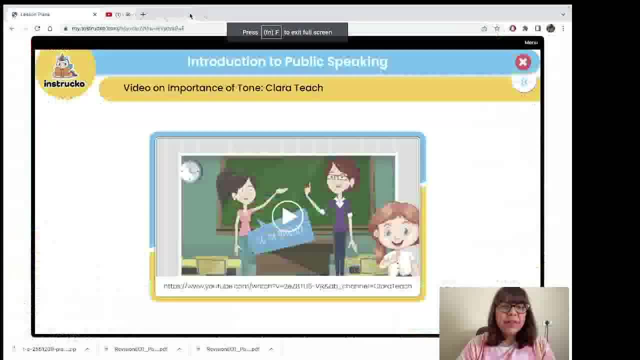 So what did all of you think of that video? So a very, very important fact, a very important point was pointed out in this video: that you know your tone of voice should match what you're feeling at that moment. right, Suppose you're sounding, you're feeling very. 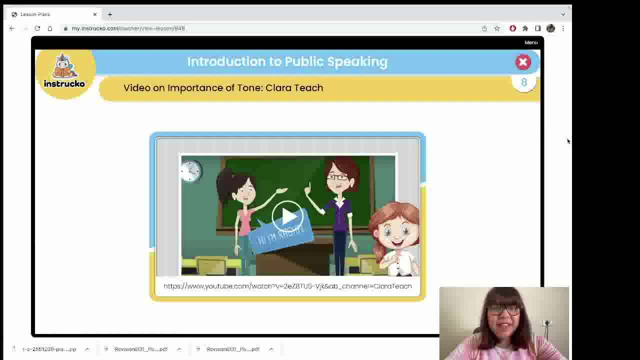 upset, but then you don't sound upset, You sound happy. Will you get the kind of reaction that you expect from yourself? Will you get the kind of reaction that you expect from you? Will you get the kind of reaction that you expect from yourself? Will you get the?